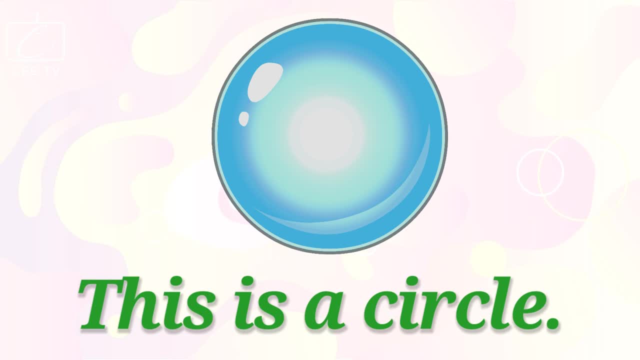 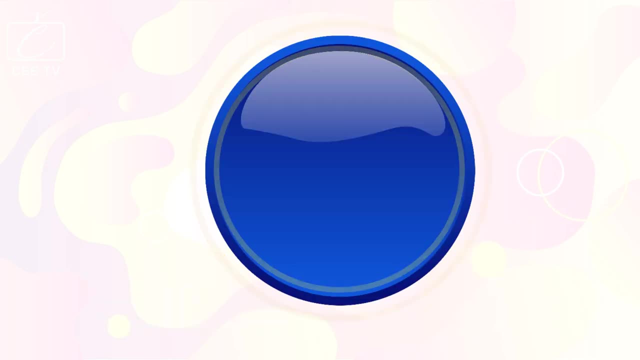 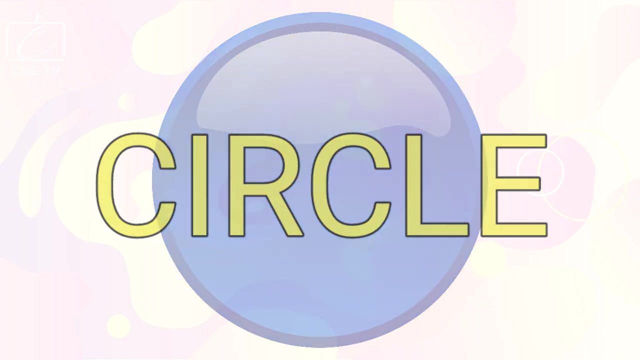 This is a circle. You are correct, This is a circle. A circle is round. It has no corners. Circle: You are correct, This is a circle. A circle has four sides. All the sides are equal. You are correct, This is a circle. 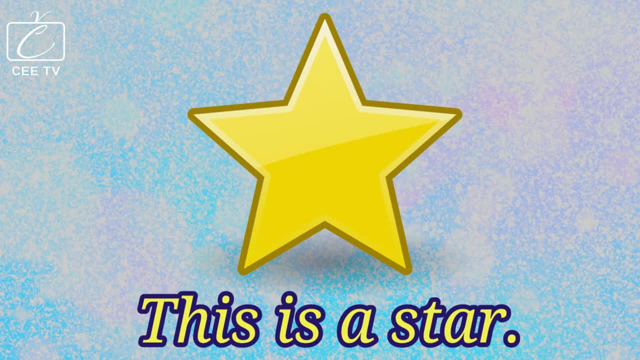 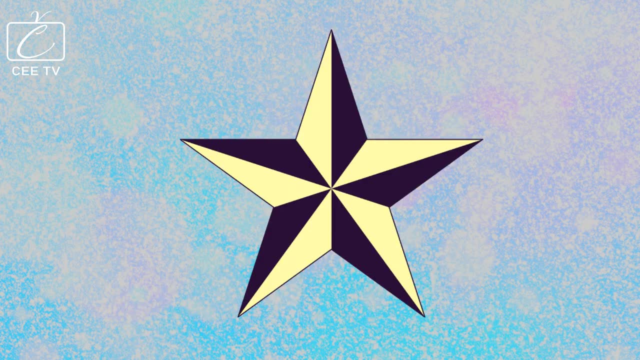 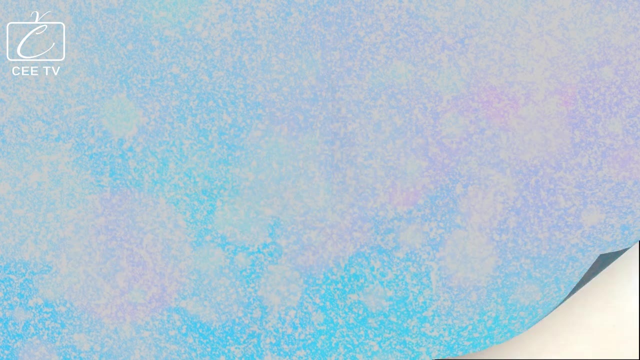 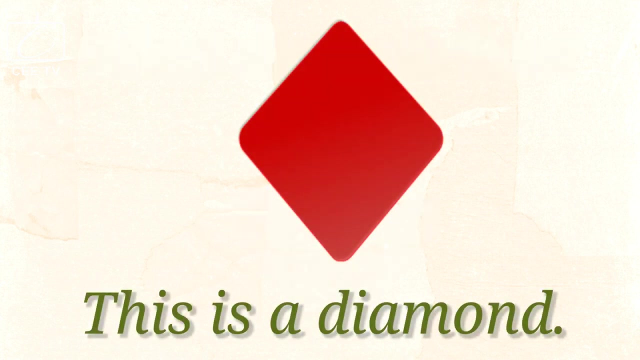 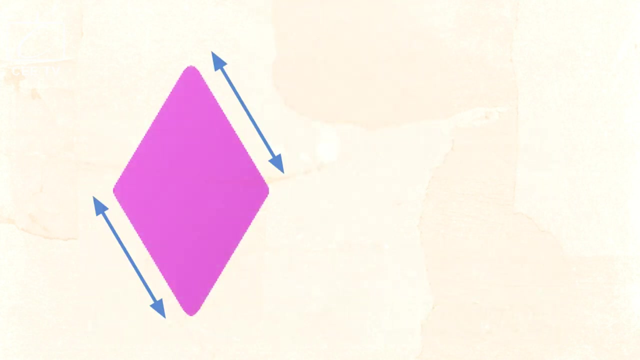 This is a star. This is a star. Great job. Yes, this is a star. A star is a shape with five points. Star, What shape is this? This is a diamond. You got it right: This is a diamond. A diamond has four sides. 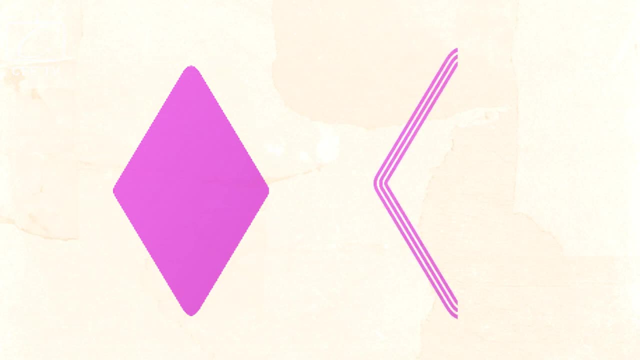 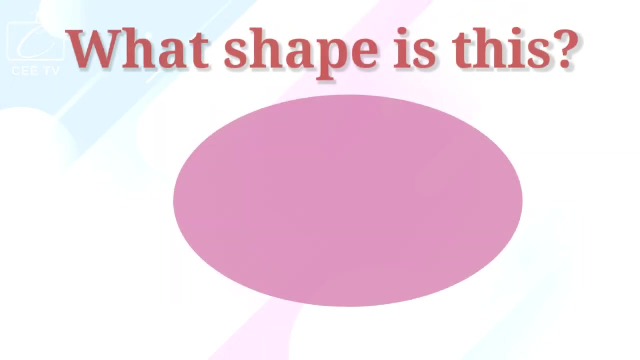 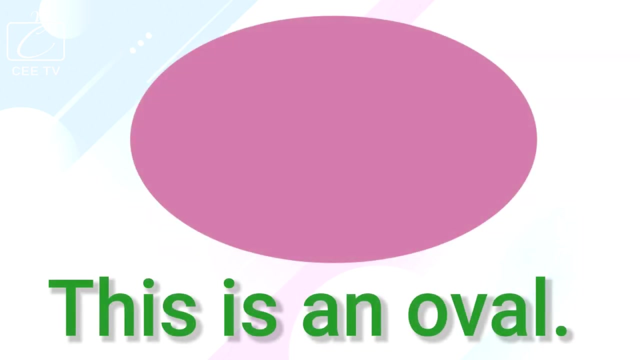 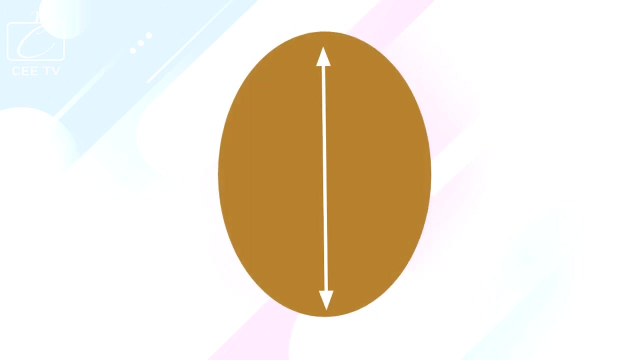 Its opposite sides are parallel and its opposite angles are equal. Diamond, What shape is this? This is an oval. Very good, This is an oval. An oval is like a circle, but is slightly elongated. It has an outline of an N. 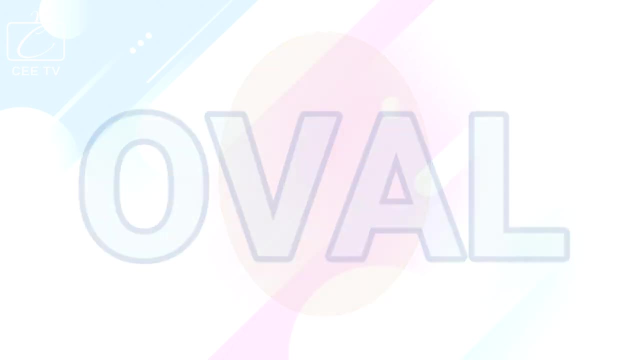 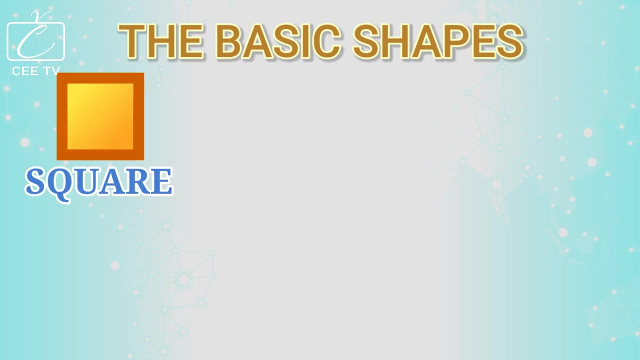 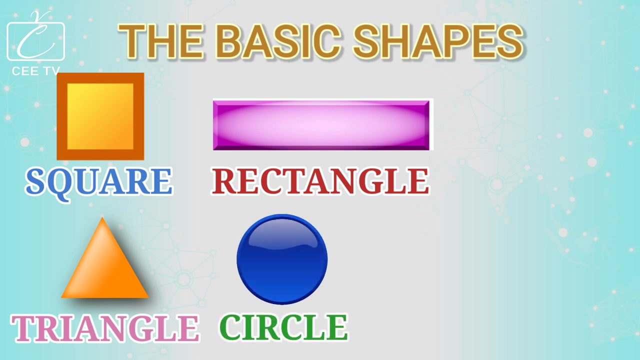 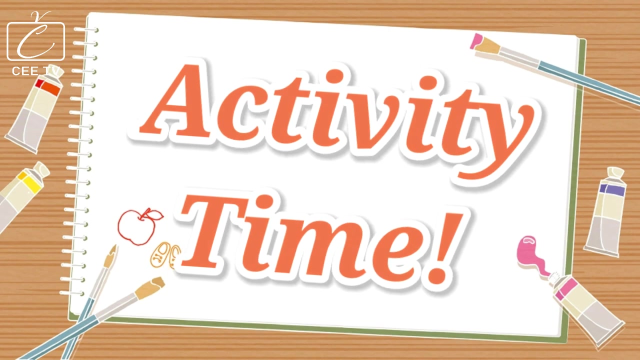 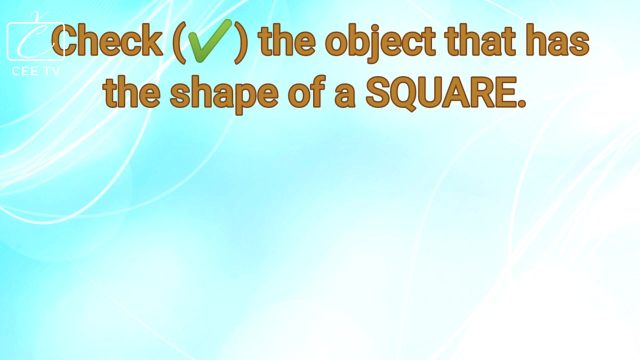 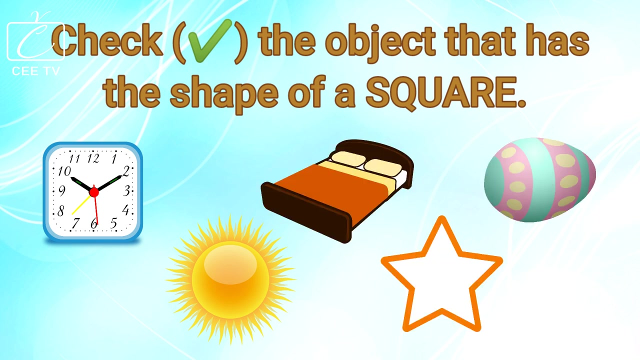 Oval. Let's learn again the basic shapes: Square, Square, Triangle, Triangle, Rectangle, Rectangle, Circle, Circle, Star, Star, Star, Diamond, Diamond, Oval, Oval, Oval, Oval, Activity, time Oval. Check the object that has the shape of a square, Square, Square. The clock has the shape of a square. 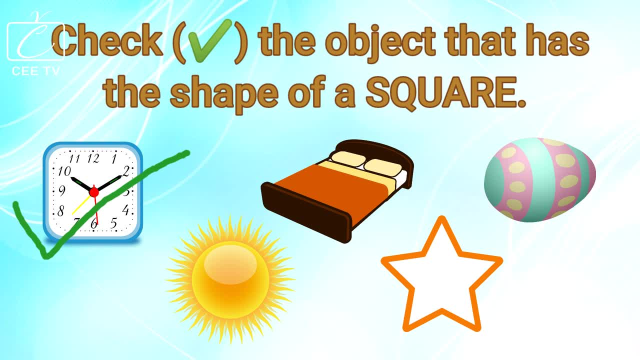 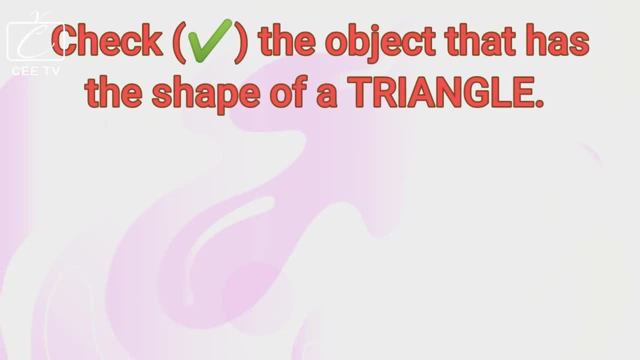 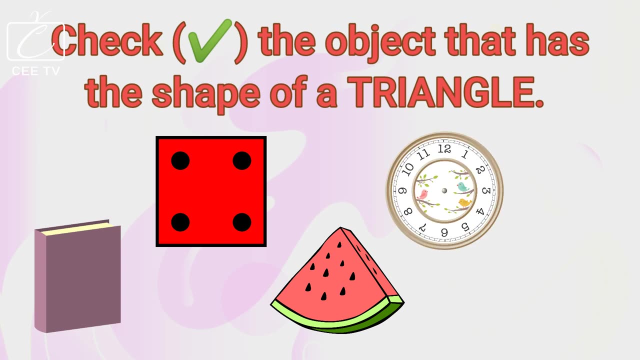 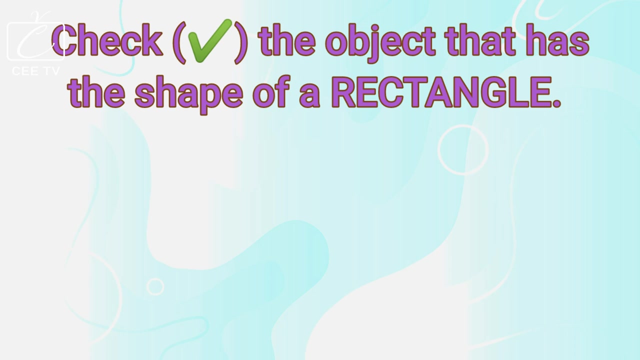 Great job. The clock has the shape of a square. Check the object that has the shape of a triangle. The watermelon has the shape of a triangle. Excellent, The watermelon has the shape of a triangle. Check the object that has the shape of a rectangle. 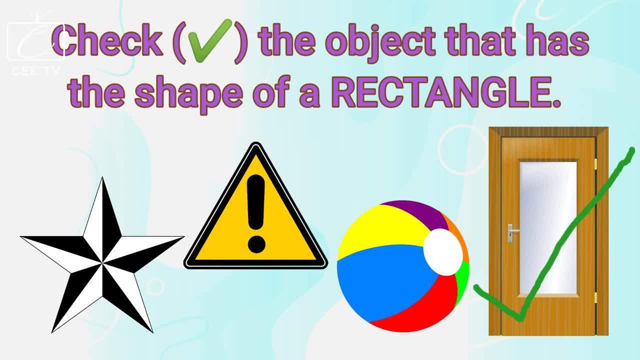 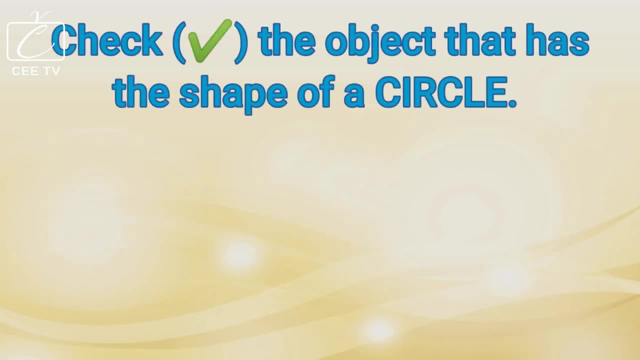 The door has the shape of a rectangle. Fantastic, You are correct, The door has the shape of a rectangle. Check the object that has the shape of a circle: The orange has the shape of a circle. Very good, The orange has the shape of a circle. 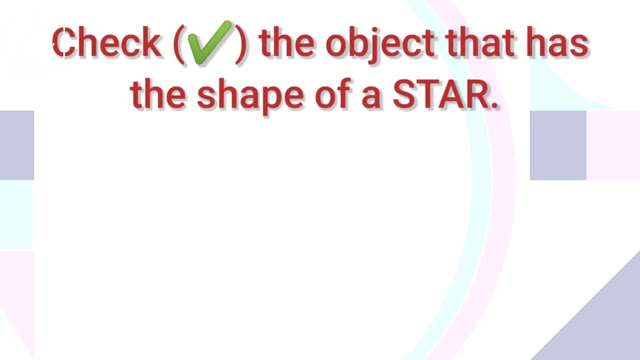 Check the object that has the shape of a circle Very good. Check the object that has the shape of a circle: Very good. The orange has the shape of a circle Very good. The orange has the shape of a circle Very good. 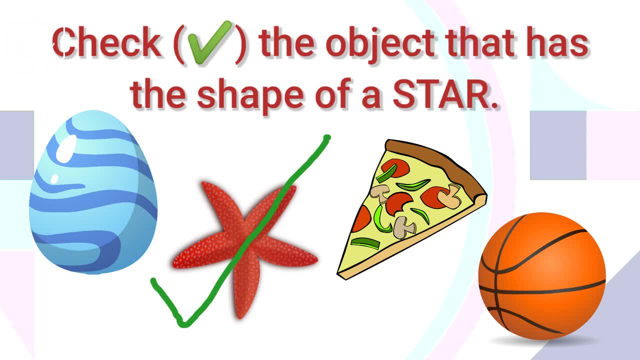 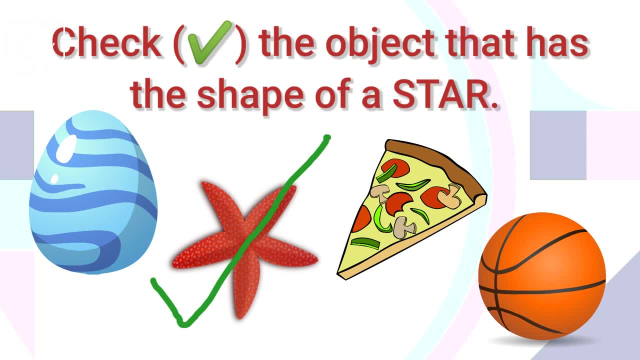 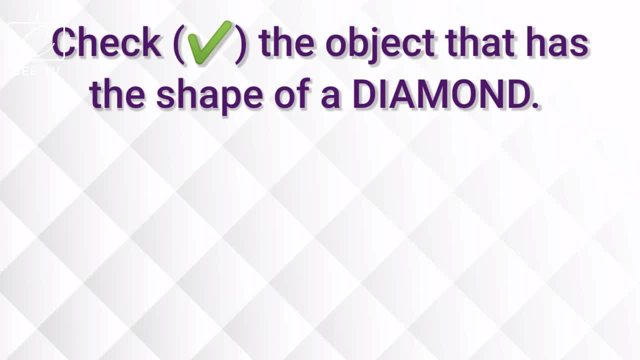 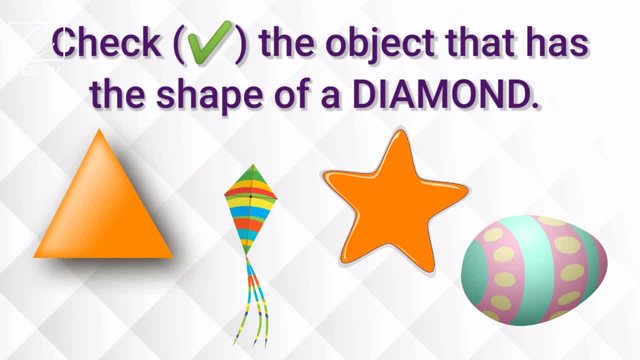 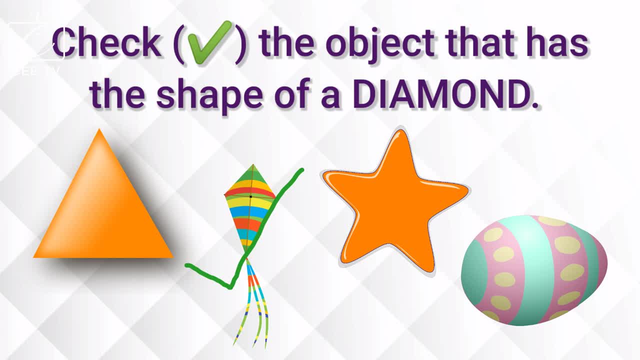